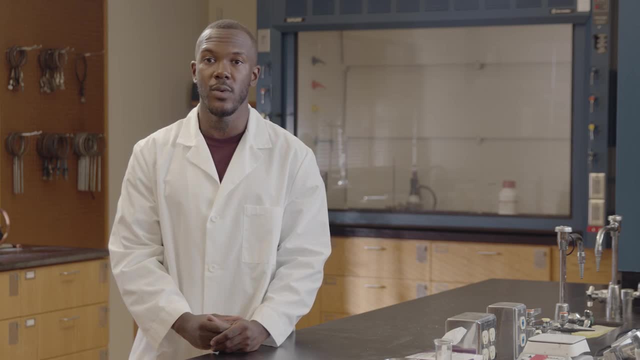 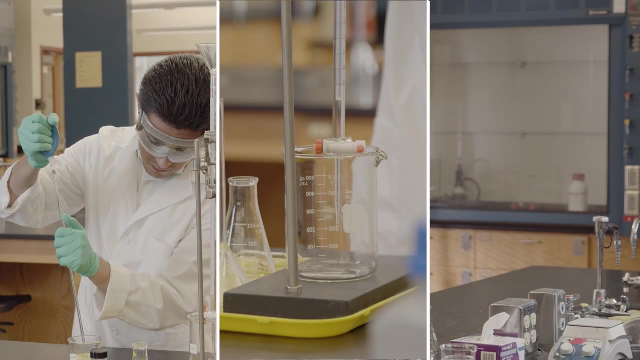 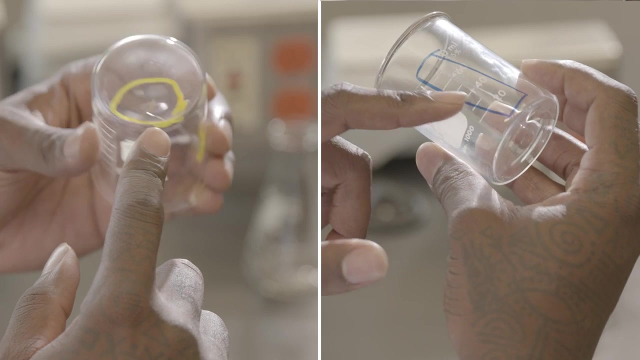 Now let's look at two common lab techniques and how to reduce the risks associated with them. Titrations require the use of glassware. When using glassware, be sure to inspect it for star fractures or hairline cracks. Simply bumping or heating a flask or beaker with a hairline crack can cause it to break. 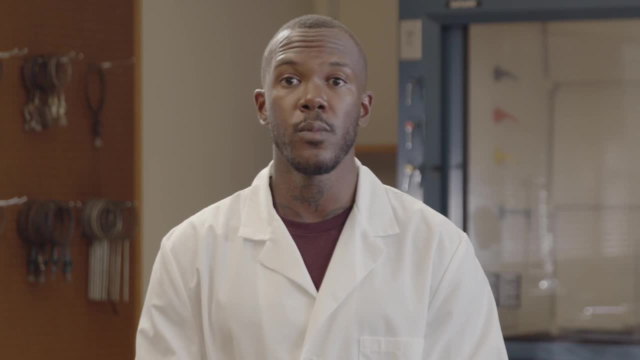 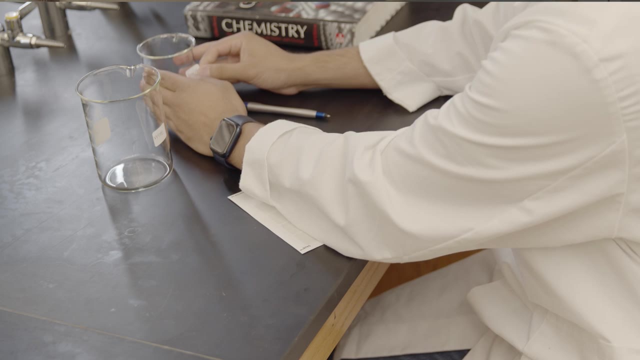 Many solutions and solvents look just like water, so it's important to temporarily label beakers and flasks while in use. Unmarked containers can cause confusion, which could lead to you or someone else mixing the wrong chemicals. The titrant is a solution of known concentration added to the burette. 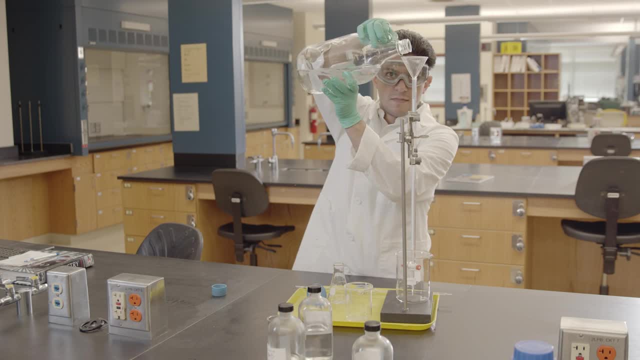 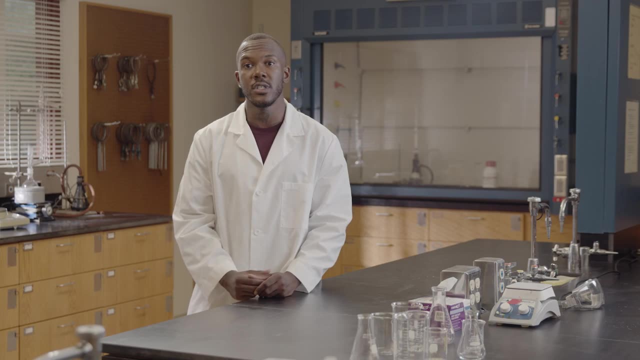 Pouring from a reagent bottle can be awkward and increases the risk of a spill. It's best to pour from a small beaker over which you have more control. After estimating how much titrant is needed, pour about 10% extra into a labeled beaker. 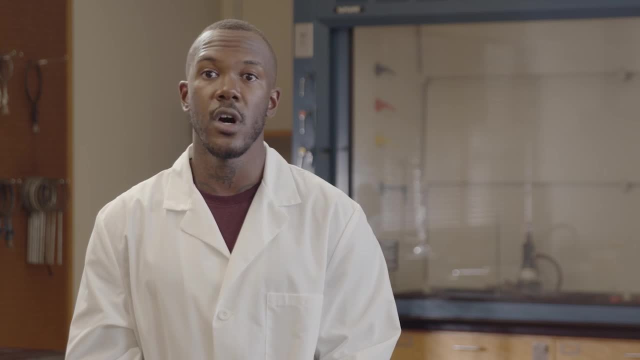 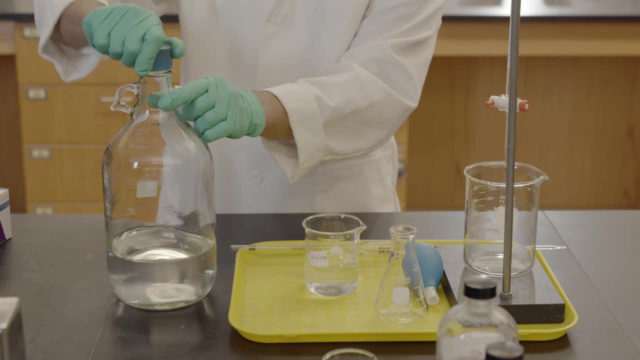 Be careful not to let drips run down the side of the reagent bottle. This can cause a minor spill and also leaves drops on the bottle that the next person might touch. Wipe off any drips and completely replace the lid. When pouring the titrant into the burette, keep the top of the burette just below eye. 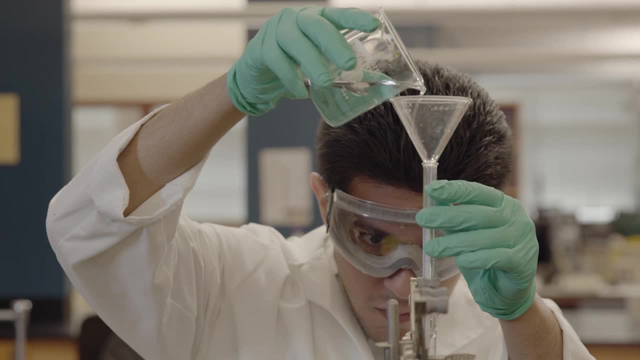 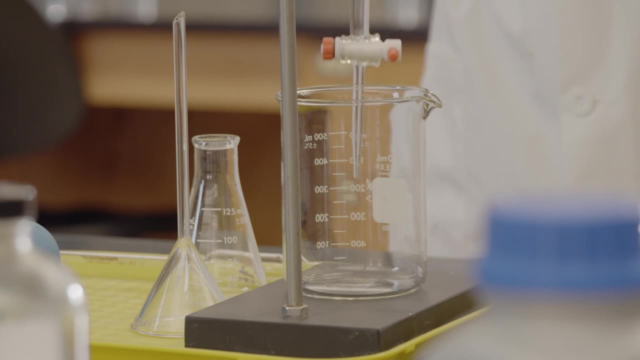 level. This makes it easier to watch the pouring process. Be sure to pour slowly, especially if using a funnel, to make sure you don't exceed the volume of the burette. Place a large beaker under the tip of the burette to catch any spills. 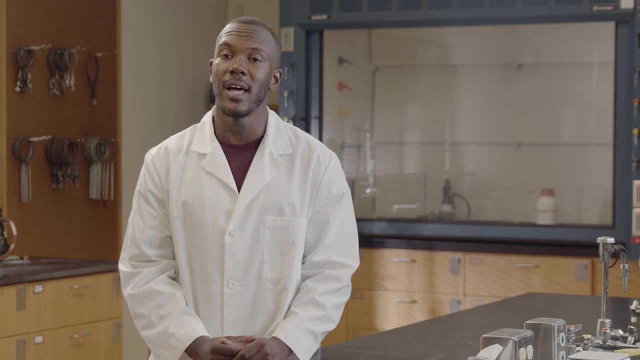 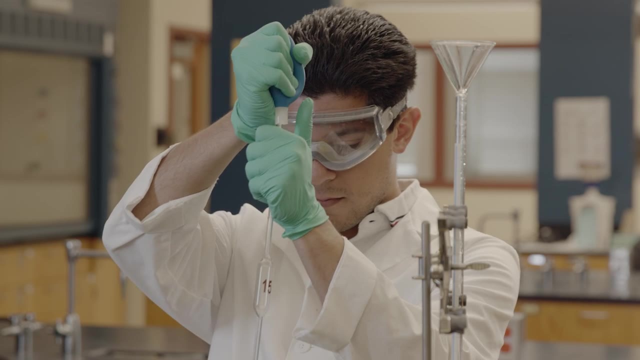 A pipette is often used to measure a known amount of the solution to be analyzed, also called the analyte. To safely connect the pipette to the bulb, grasp the pipette close to the end and gently insert it into the bulb. Applying too much force can break the pipette, which can result in serious injury. 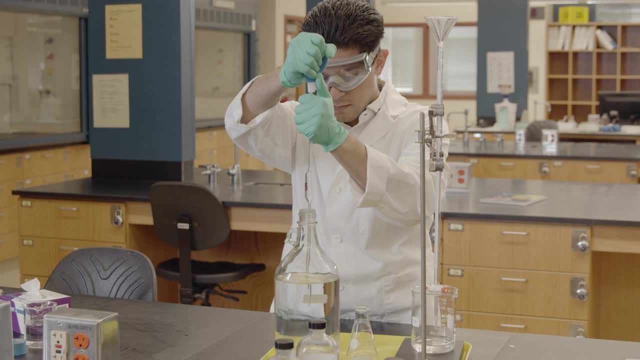 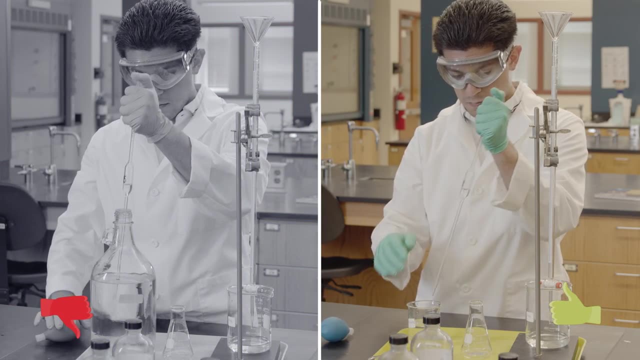 Ow. It's important not to place the pipette into the bottle of stock solution to avoid contamination. Obtain 10% more than you need in your beaker and pipette from the beaker. Any excess should not go back into the stock solution again to avoid contamination. 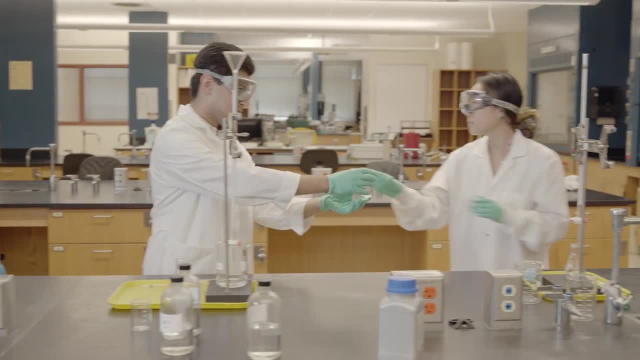 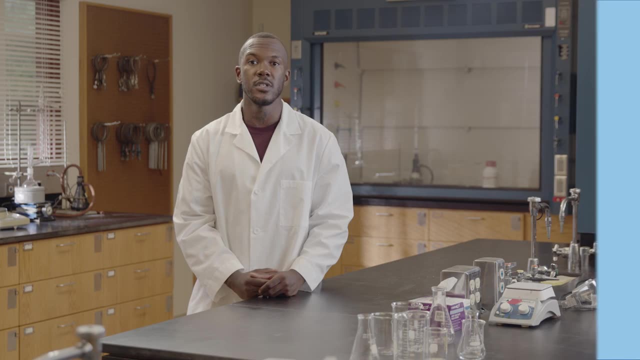 If you have leftover titrant or analyte, you can offer to share this with a lab mate. Otherwise, dispose of it in the proper waste container. Chemical synthesis is another common lab experiment with both chemical and procedural hazards. A common process is to make sure that the solution is in the right place. 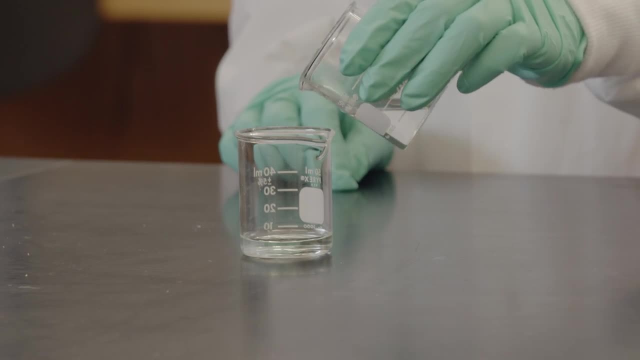 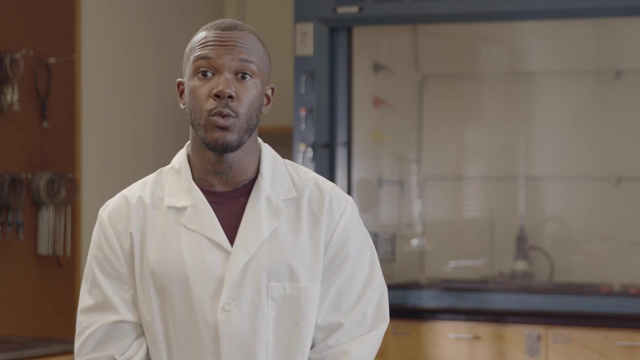 The common process is to mix solutions of chemicals, heat and stir the mixture to produce a precipitate and isolate the precipitate by filtration. To start a chemical synthesis you may need to weigh your reagents. Take your reaction flask and notebook to the balance. 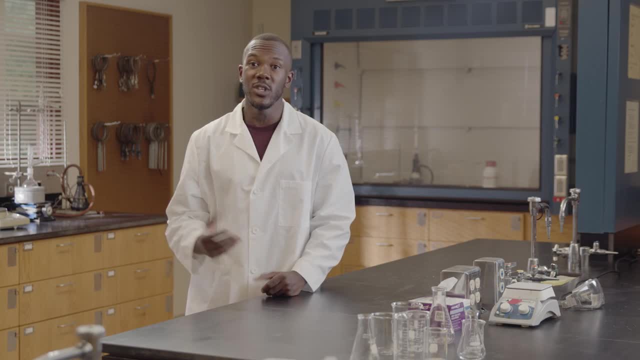 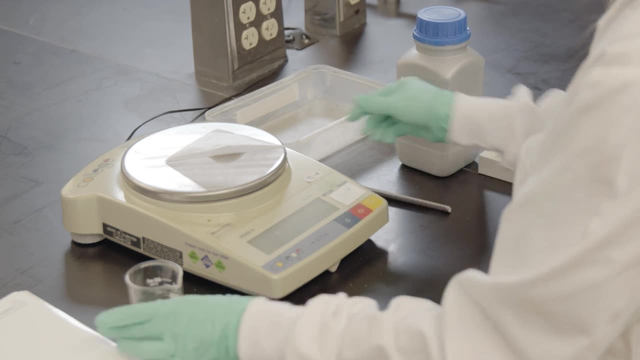 Obtain the desired amount of each solid in small increments. If you get too much at first, put the excess into a waste container to avoid possible contamination of the original reagent. If you spill any solid at the balance, clean this up immediately and put the spilled solid. 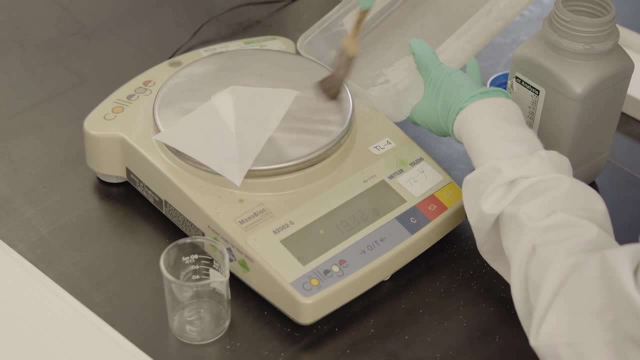 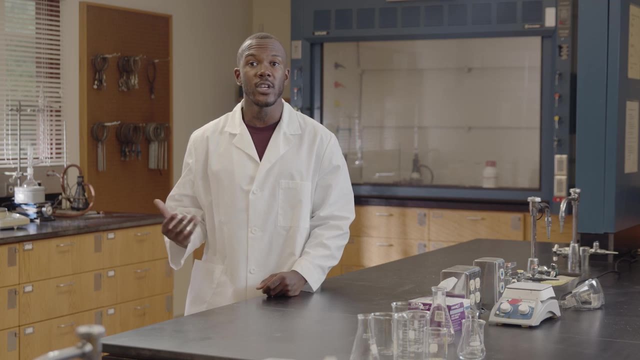 into a waste container. Place the weighed solids into the flask immediately, rather than trying to walk through a crowded lab with the solids on weighing paper. For reaction in water, heating is usually done on a hot plate. When using any electrical equipment, it's best to check the cord for frayed connections. 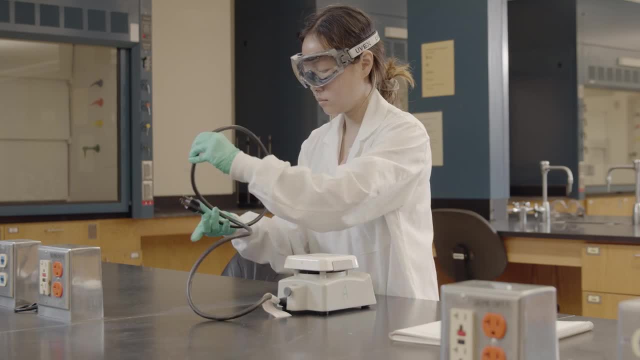 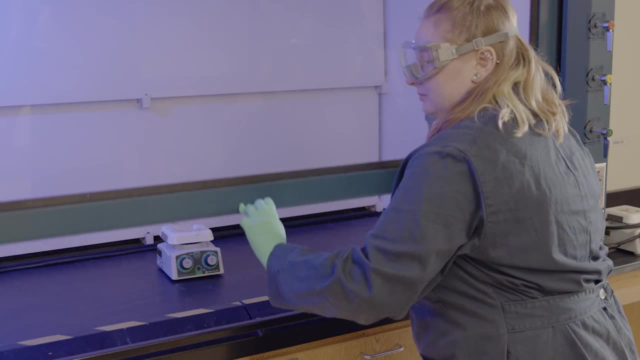 Keep the cord off the hot surface and set the hot plate on a dry surface. If there is any chance a hazardous gas will be produced. conduct the reaction in a hood, where the gas will be quickly removed. Hoods reactions that use a flammable organic solvent too. 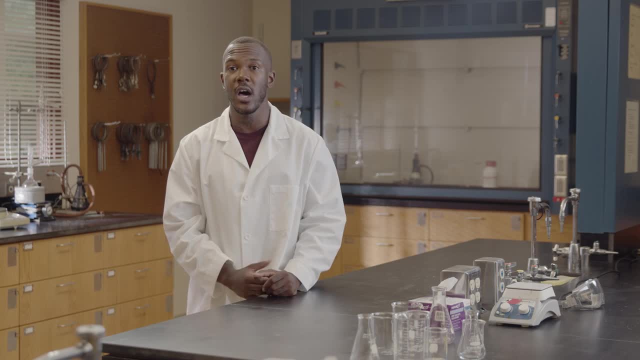 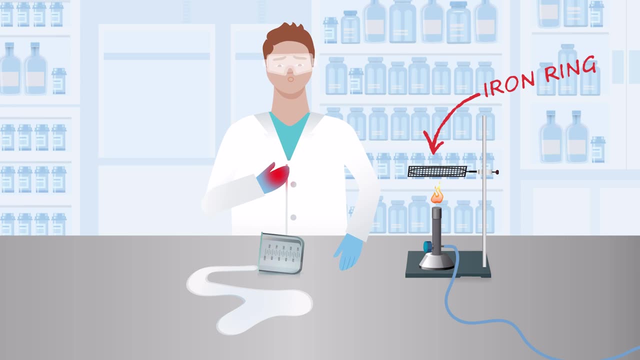 A properly functioning hood will minimize the chance that the organic vapor comes in contact with the heat source. Hot glass looks just like cold glass and a hot iron ring looks like a cold iron ring. Handle any hot object with beaker tongs or crucible tongs. 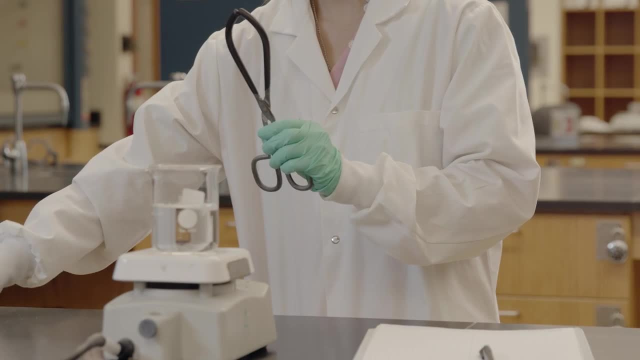 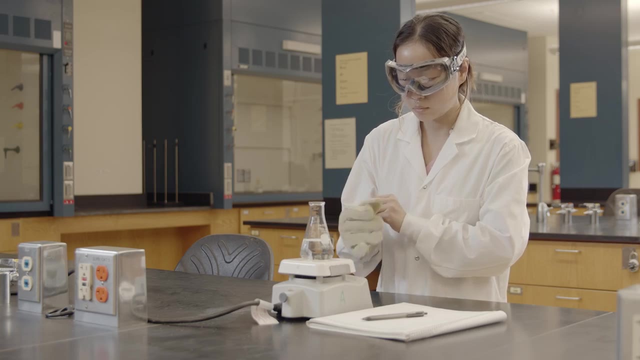 These are not interchangeable and using the wrong tool can lead to dropping the container, breaking it or spilling the contents. Sometimes a hot object is best handled by special heat-resistant gloves. Hot beakers or flasks should only be placed on a hot plate. 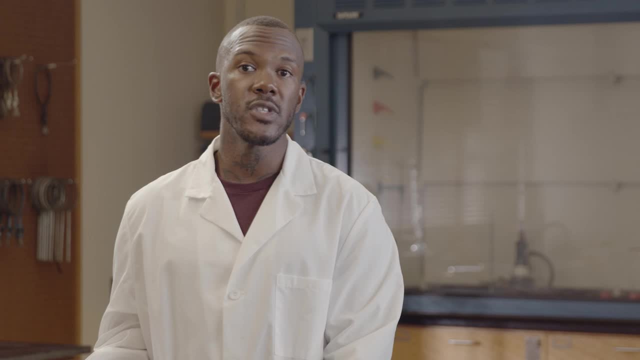 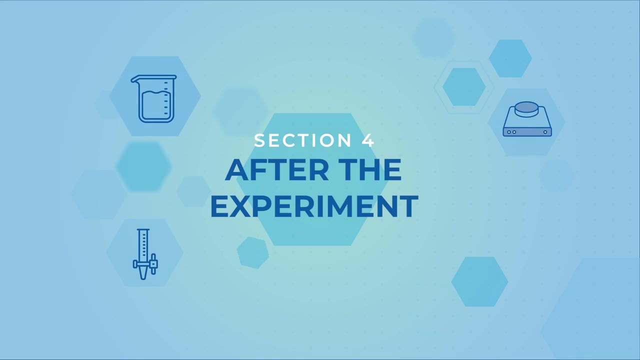 They should only be placed on surfaces that are heat-resistant. Spills of any solids or liquids should be cleaned up immediately. Typically, your lab instructor will take care of this or show you how to do so. As noted earlier, at the end of an experiment you often have leftover solids, solvents.